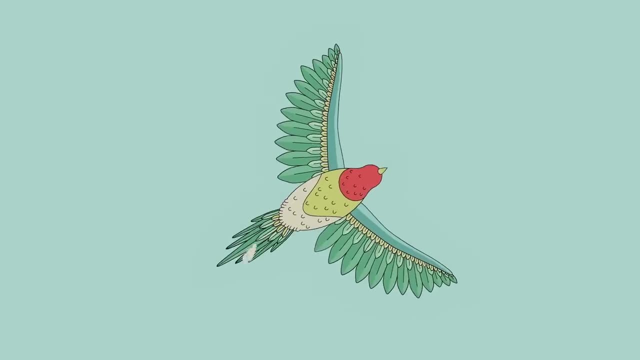 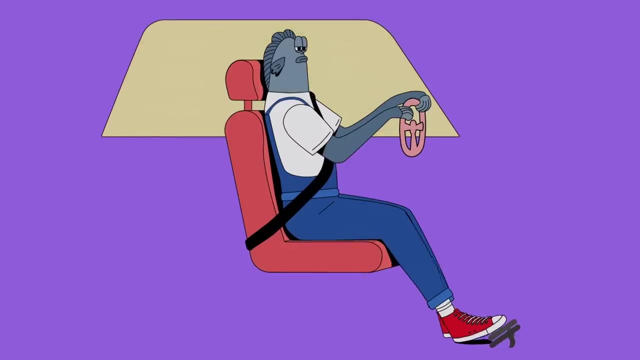 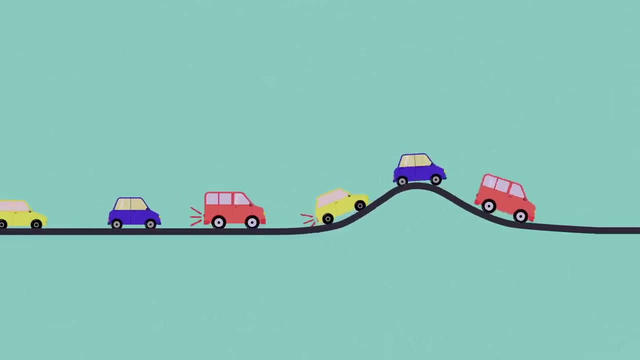 In this dense but flowing traffic it only takes a minor disturbance to set off the chain of events that causes a traffic jam. Say, one driver brakes slightly, Each successive driver then brakes a little more strongly, creating a wave of brake lights that propagates backward through the cars on the road. 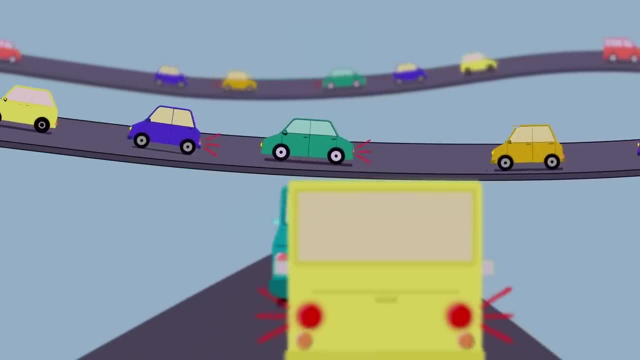 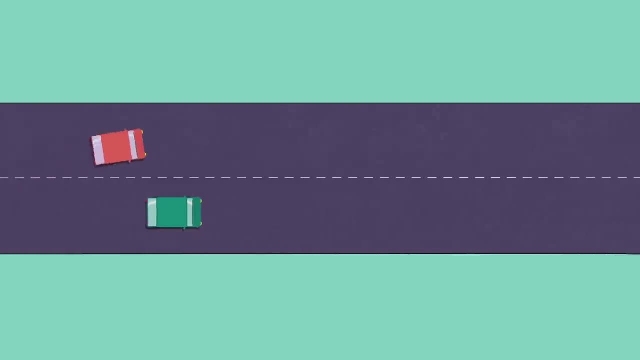 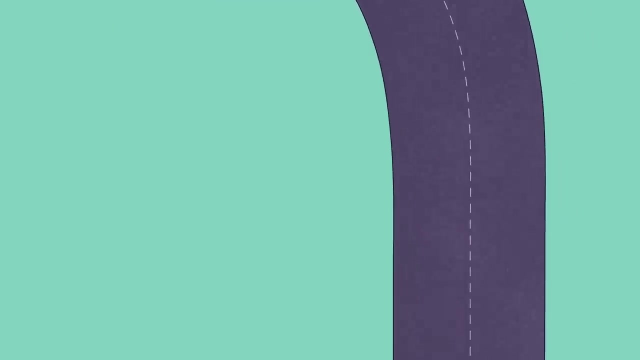 These stop-and-go waves can travel along a highway for miles With a low density of cars on the road. traffic flows smoothly because small disturbances, like individual cars changing lanes or slowing down at a curve, are absorbed by other drivers' adjustments. But once the number of cars on the road exceeds a critical density, 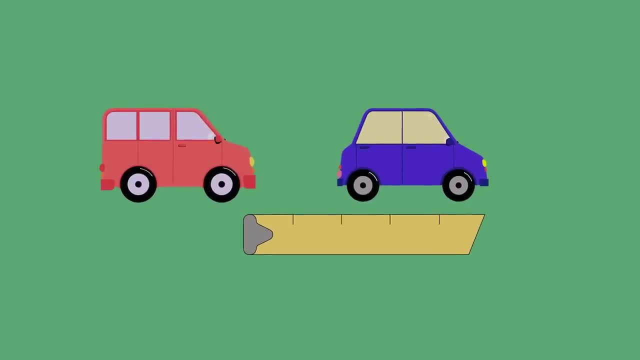 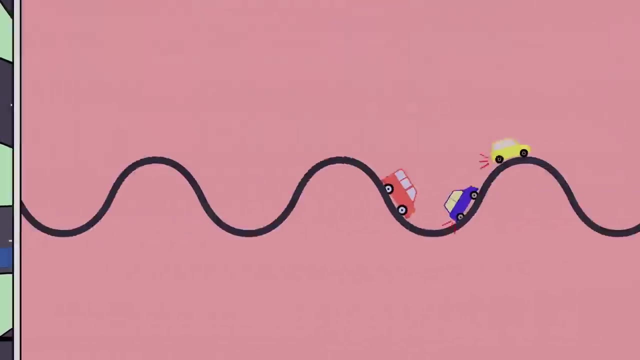 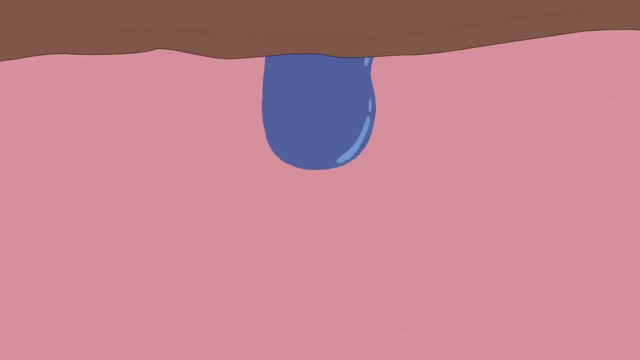 generally, when cars are spaced less than 35 meters apart, the system's behavior changes dramatically. It begins to display dynamic instability, meaning small disturbances are amplified. Dynamic instability isn't unique to phantom traffic jams. It's also responsible for raindrops, sand dunes, cloud patterns and more. 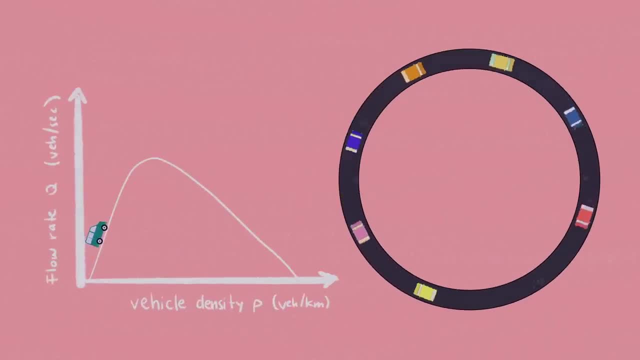 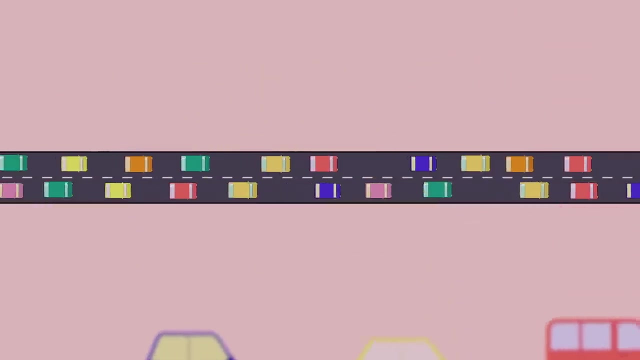 The instability is a positive feedback loop. Above the critical density, any additional vehicle reduces the number of cars per second passing through a given point on the road. This in turn means it takes longer for a local pileup to move out of a section of the road. increasing vehicle density even more, which eventually adds up to stop-and-go traffic. Drivers tend not to realize they need to brake far in advance of a traffic jam, which means they end up having to brake harder to avoid a collision. This strengthens the wave of braking from vehicle to vehicle. 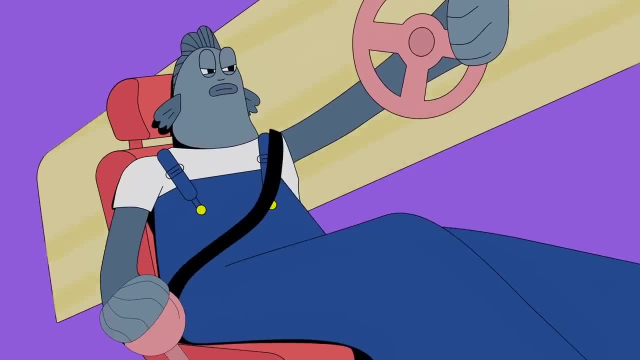 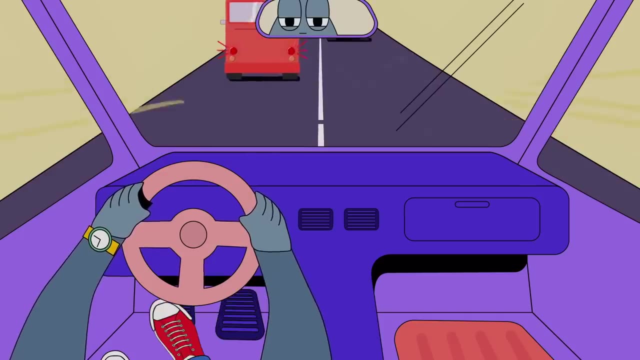 What's more, drivers tend to accelerate too rapidly out of a slowdown, meaning they try to drive faster than the average flow of traffic downstream of them. Then they have to brake again, eventually producing another feedback loop that causes more stop-and-go traffic. 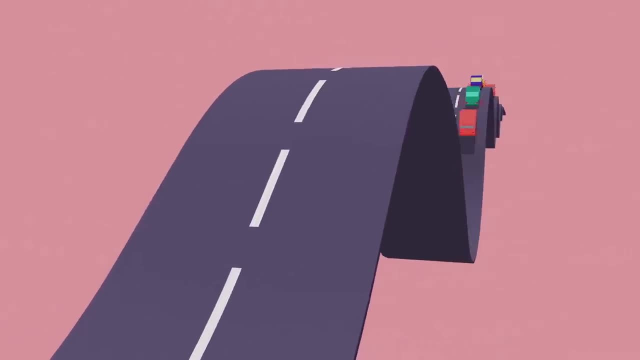 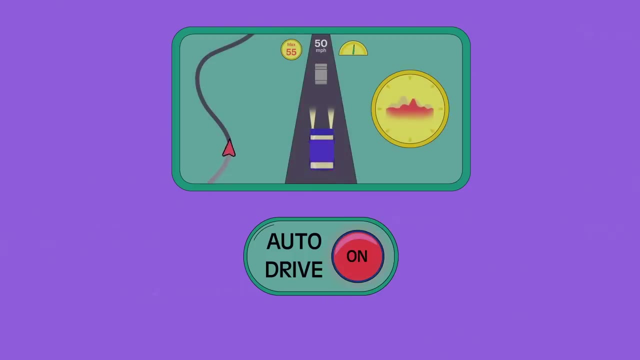 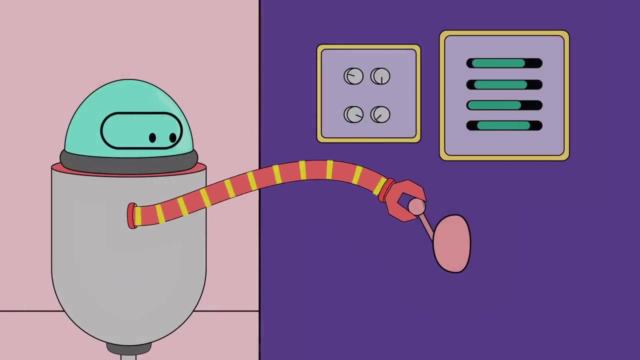 In both cases, drivers make traffic worse simply because they don't have a good sense of the conditions ahead of them. Self-driving cars equipped with data on traffic conditions ahead from connected vehicles or roadway sensors might be able to counteract phantom traffic in real time. 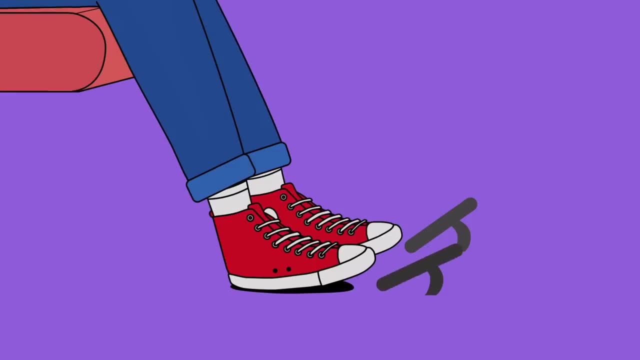 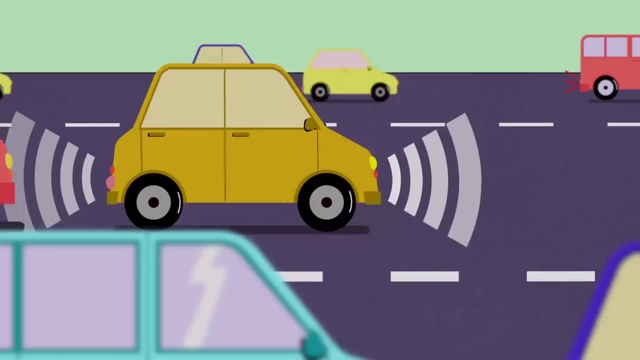 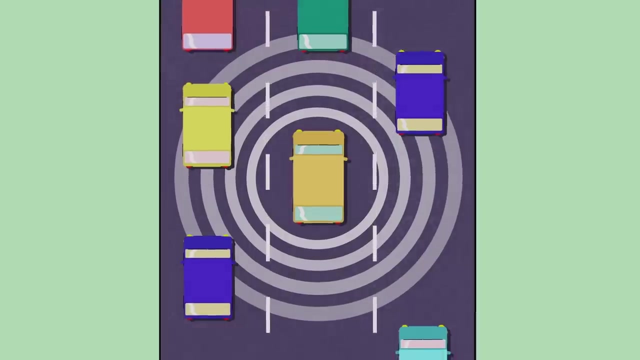 These vehicles would maintain a uniform speed safety permitting that matches the average speed of the overall flow, preventing traffic waves from forming. In situations where there's already a traffic wave, the automated vehicle would be able to anticipate it braking sooner and more gradually than a human driver.